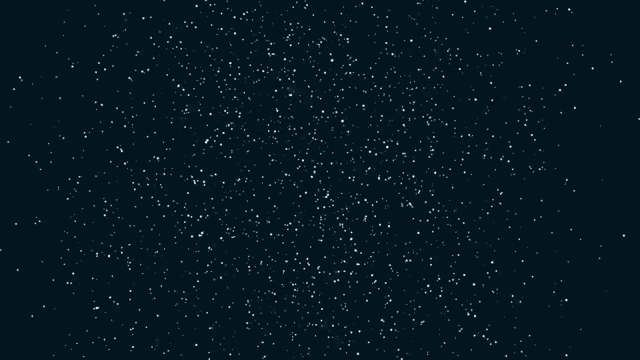 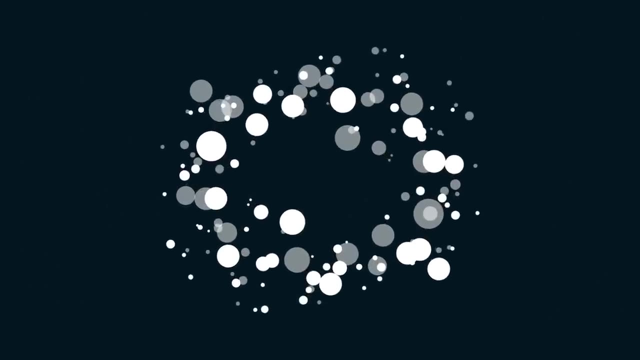 structures like galaxies are torn apart since space between the single objects expands very fast. Next, big bodies like black holes, stars and planets die. Their gravity isn't strong enough to keep them together, so they dissolve into their components. In the end, space would expand. 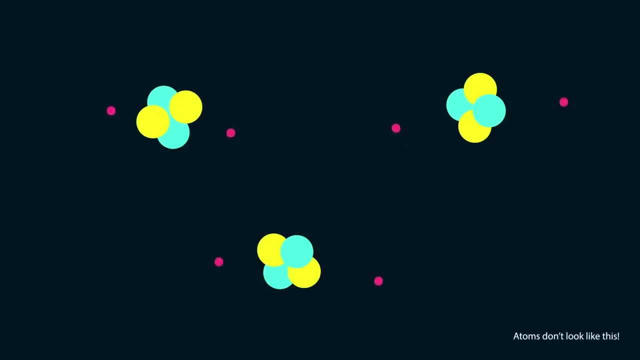 faster than the speed of light. Atoms would now be affected and they would just disband. Once space is expanding faster than light, no particle in the universe can interact with any other particle anymore. The universe would dissolve into countless lonely particles that won't be able to expand. The universe would dissolve into countless lonely particles that 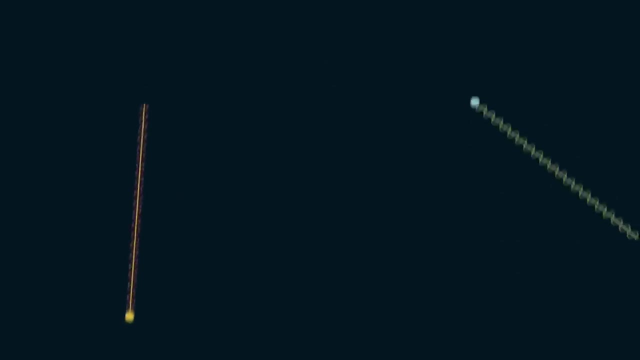 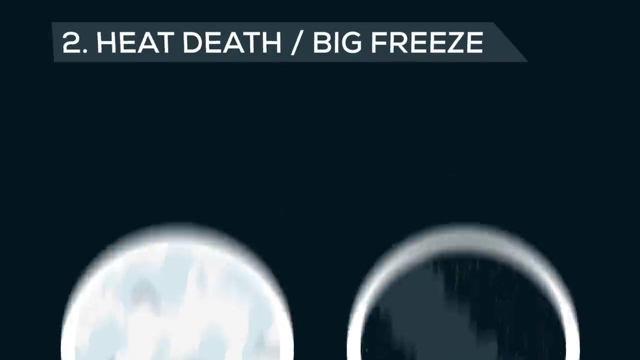 won't be able to touch anything else in a strange timeless universe. Hmm, and you thought you felt lonely. 2. Heat Death or a Big Freeze. In a nutshell, the difference between the big rip and heat death is that in a heat death scenario, 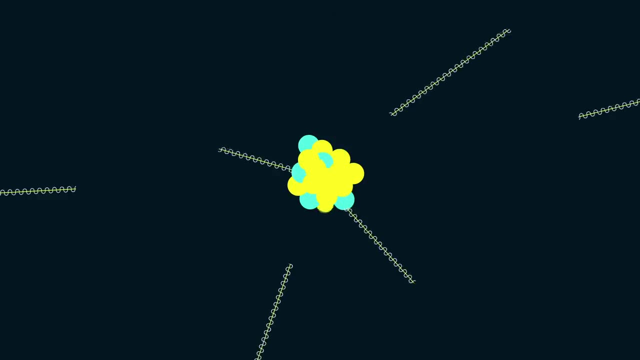 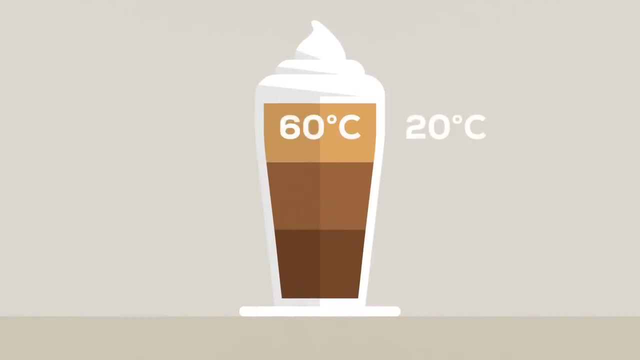 matter stays intact and is converted over an incredibly long but finite period of time into radiation, while the universe expands forever. But how does this work? Let's talk about entropy. Every system tends towards the state of highest entropy, like when we have a latte macchiato. 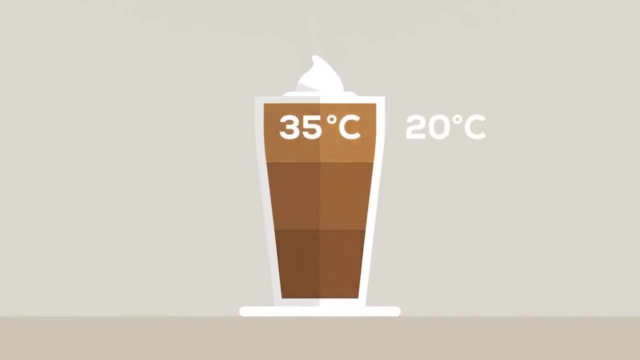 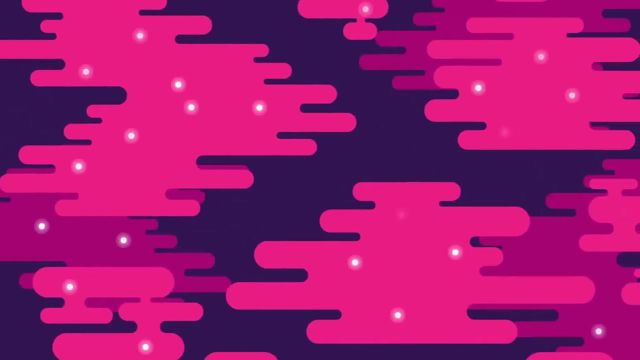 Initially it has different regions, but over time they will cool down and disintegrate until it's uniform, And this also applies to the universe. So while the universe gets bigger and bigger, matter slowly decays and spreads out. At some point- after lots of generations of stars- 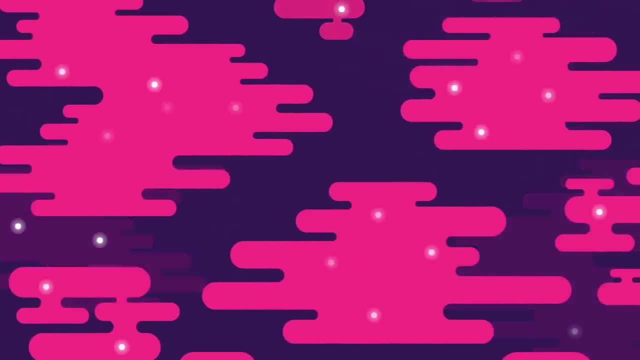 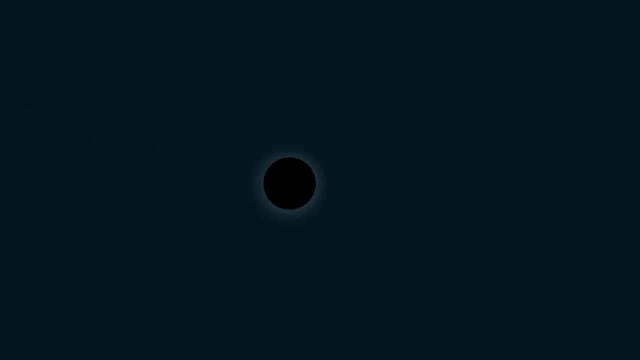 all the gas clouds necessary to form stars will be exhausted, so the universe will turn dark. The remaining suns will die, Black holes will slowly degenerate and evaporate over trillions of years due to what's known as Hawking radiation. When this process is complete, only a dilute gas of photons and light particles remains. 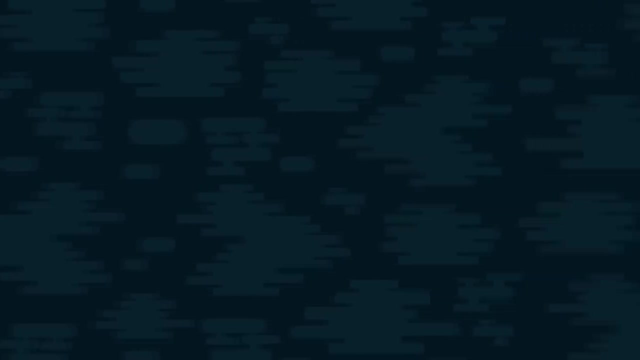 until even this decays, All activity in the universe ceases. at this point, Entropy is at its maximum And the universe will be completely empty, And the universe will be completely empty And the universe is dead forever, Unless theoretically it might be possible that after an incredibly long amount of time there might be a spontaneous entropy decrease as a result of something called quantum tunneling, leading to a new Big Bang. 3. Big Crunch and Big Bounce. This is the most uplifting scenario, If there is less dark energy than we think.